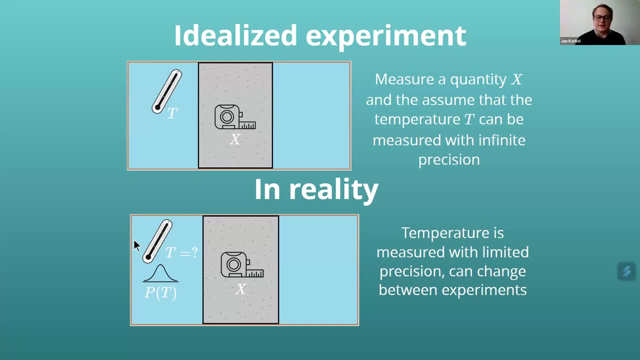 we consider that there is some uncertainty in the state of the system. So basically, if we have a trajectory or we have a set of states, we basically consider that we model it as a through the theory of probability. So there's a probability distribution over the state or 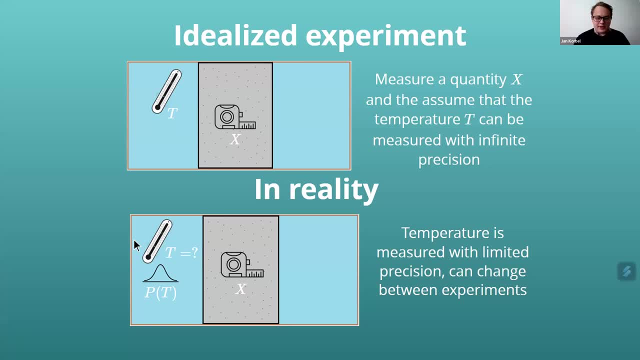 over the trajectory of the system, et cetera. But on the other hand, when we talk about the system, typically it's coupled to a heat bath or particle bath or there are some parameters of the system, And in this case we very often consider. 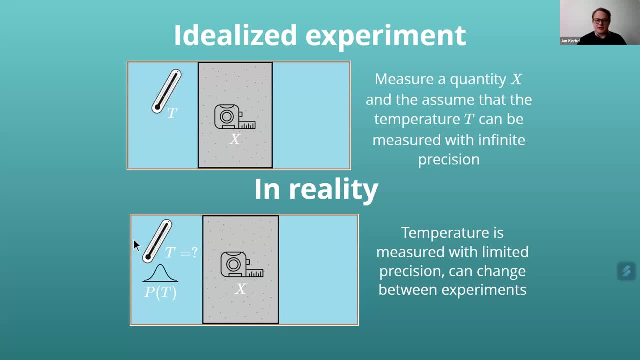 that we know these parameters like temperature, chemical potentials, et cetera, with infinite precision. So basically, what we hypothesize is that we know it exactly, And in that case we're just assuming it's a point of truth, So we might compute that. 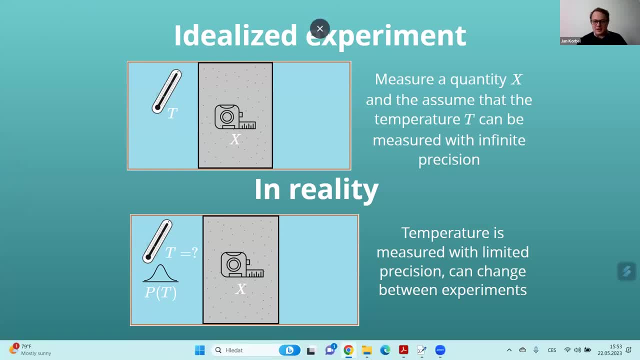 the temperature of the system is going to change and the temperature is going to change too. But in reality, what an experimenter does is that if we want to make an experiment like that, if we want to make an experiment like that, then we try to measure temperature and there is maybe 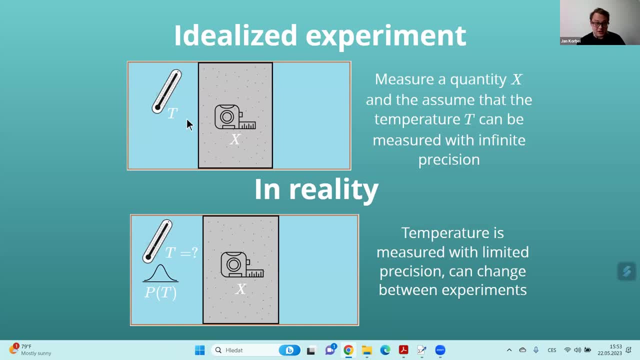 some uncertainty. or we prepare the system, And of course the device is not perfect. So we prepare the system and the temperature, for example, can slightly change. Or there are some external factors, external free-flow factors and things like that, things that we cannot, cannot affect, So that might for. 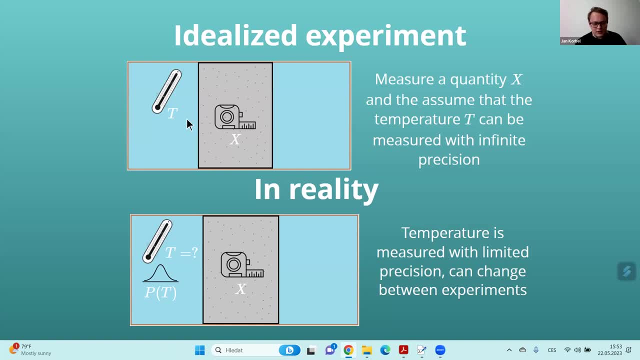 example, change the temperature of our system. Or basically, there are there are some some other external texts that that come into the game, And in this case there are two very different approaches to the system itself, where we have the knowledge that there is some uncertainty and we cannot model. 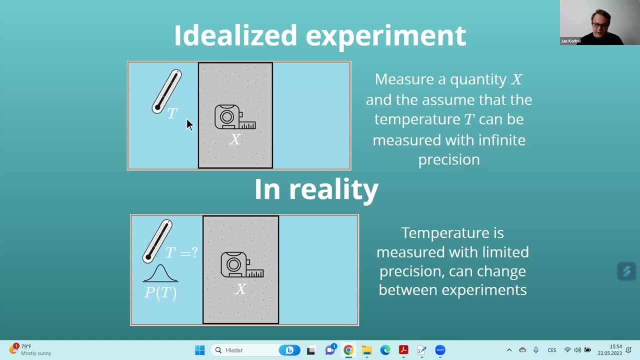 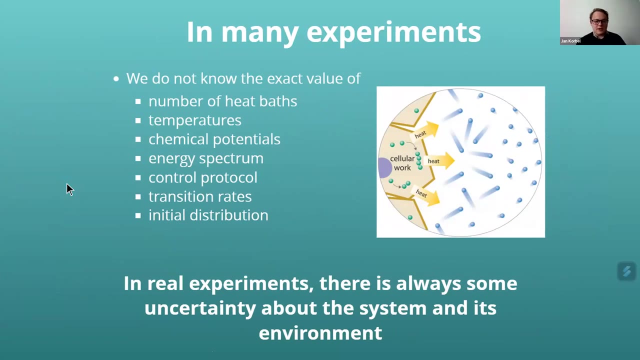 the system deterministically. On the other hand, we require that for the bath and the system parameters. we have to know them exactly And in our case, what we considered is that, as a typical experimenters, as typical experimenters, we do not know the. 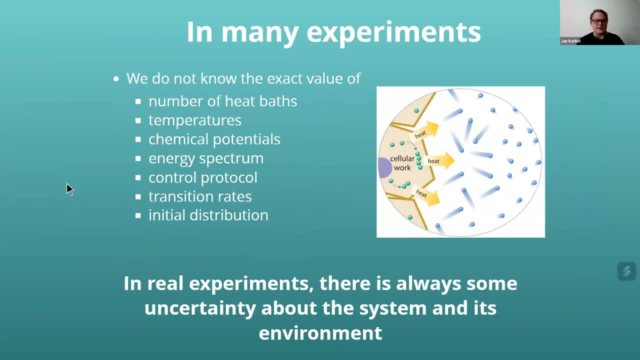 exact value of many things- number of heat, baths, temperatures, chemical potentials, energy spectrum or control protocols, transition rates, initial distributions- and there might be various reasons for it, But in general this is something that is worth investigating, also from the practical point of view that 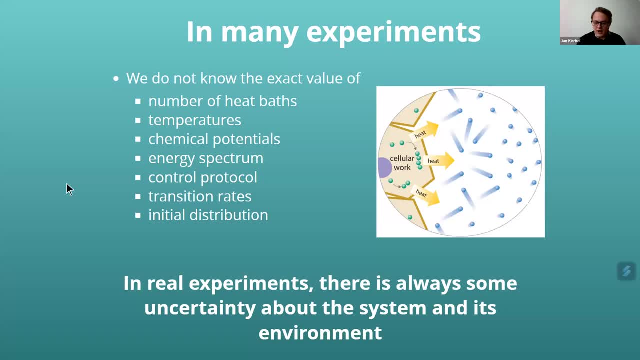 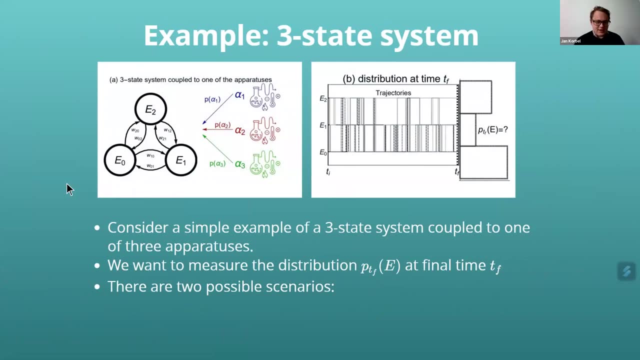 there are some uncertainties about the system and its environment, And let's start a simple example. So let's have a system that has three states And let's say that the system evolves Stochastically, so there are some transition rates between three states, let's say with different energies: E0, E1, E2.. 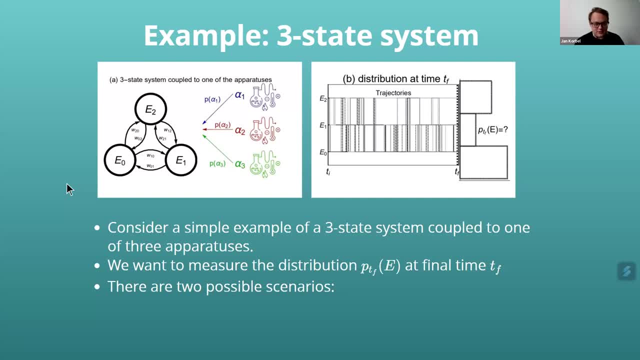 And then we say we couple the systems to three apparatuses And these apparatuses affect the exact form of the transition rates. And now the question is: do we know this Or can we somehow say something about the apparatus? So now we want to measure the distribution at final time and 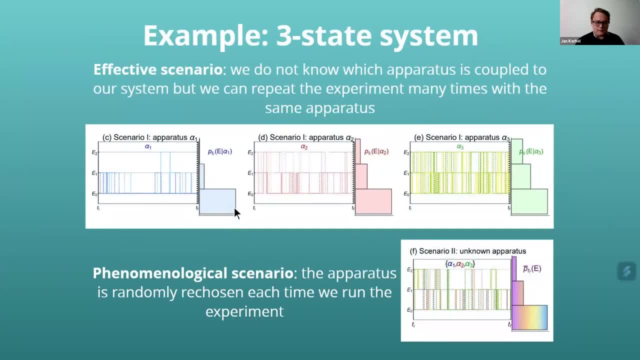 there are two possible scenarios. So either we have the apparatus, then we can run the experiment many times. So we run the experiment and we want to measure, for example, a probability distribution at time tf. So what we do is that basically let the experiment run, stop it at tf, measure a. 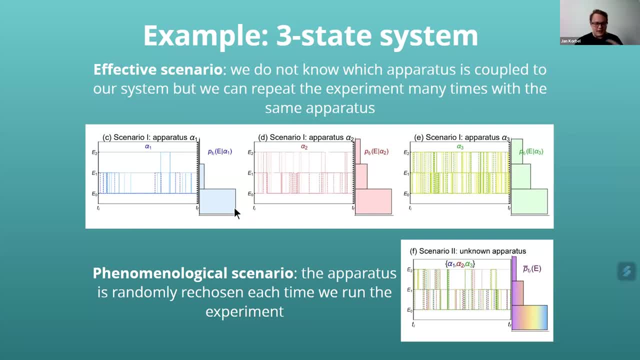 position of particle. repeat the experiment and do it so many times that, until we get a decent estimate of the probability distribution And in case that, if we know that the apparatus is the same for each run, then what we can measure is this conditional distribution of, for example, energy, given the 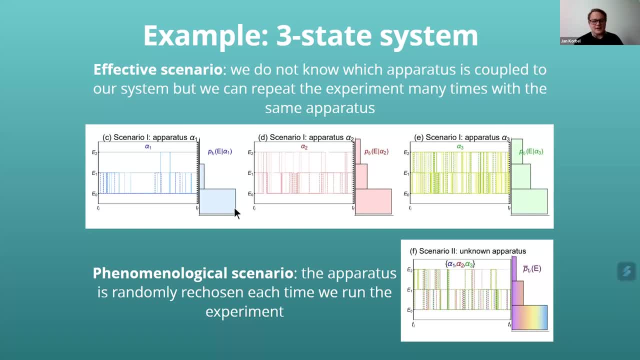 given the apparatus, But sometimes we- and this is what we call effective scenario- And then we can do many measurements for the apparatus alpha one, many measurements for the apparatus alpha two, many measurements for the apparatus alpha three, And then for each of these we can measure this: 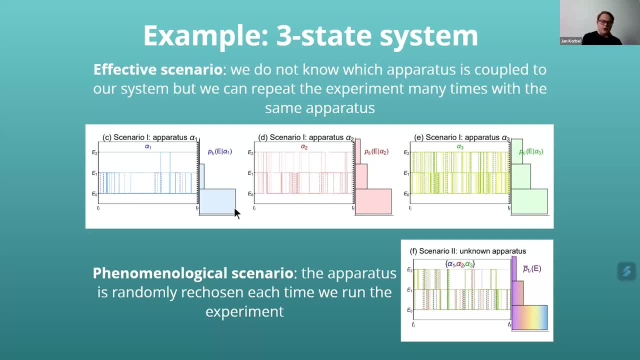 probability distribution And then, if we want, we can also make an average over the apparatuses and make the average value over the each apparatus, averaging over the probability distribution of each apparatus. But very often what happens is that we don't know exactly the apparatus and the 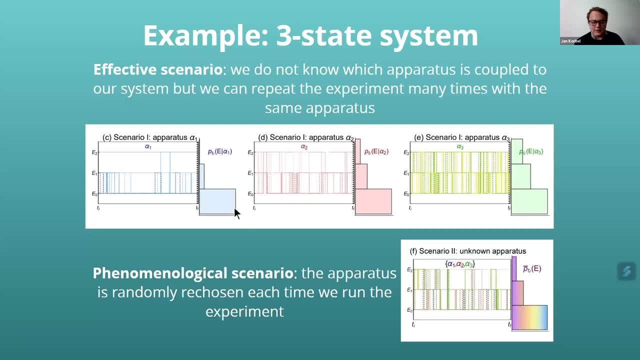 each apparatus is randomly chosen. each time you run the experiment, the temperature slightly changes, because the sun is shining on our experiment, or there is some air conditioning that changes the temperature, something that we don't know, And then, in this case, we can only measure the, let's say, the, 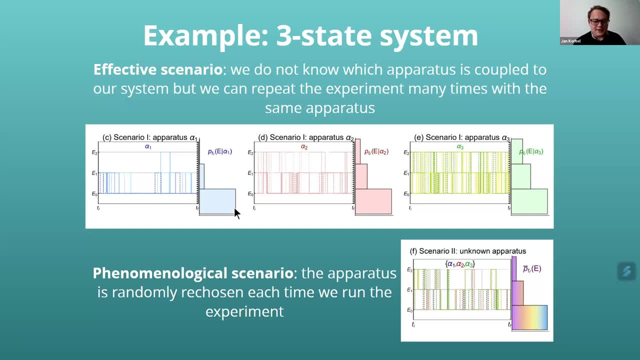 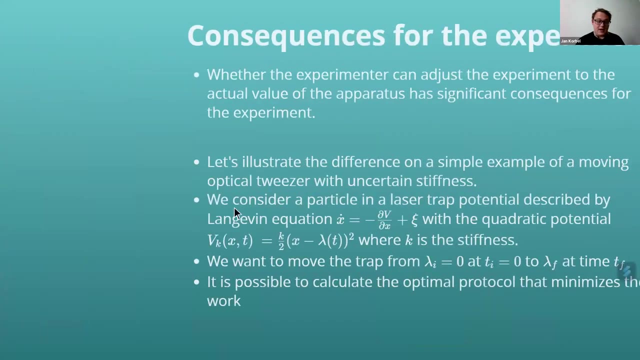 the average of all the apparatuses at once, And this is what we call phenomenological scenario, And one can think: okay, so in one case I can measure the quantity for each apparatus. In one case I cannot. But the question is: does it change the experiment? And the answer is yes. 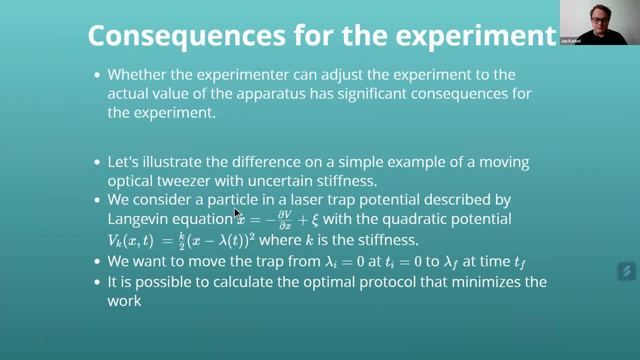 it might change the experiment. So because in the case where we know that we are coupled to a single apparatus and then we can adopt our control protocol, for example, So then we can basically adjust the experiment to the conditions we have. So let's say we have a simple example of a moving optical. 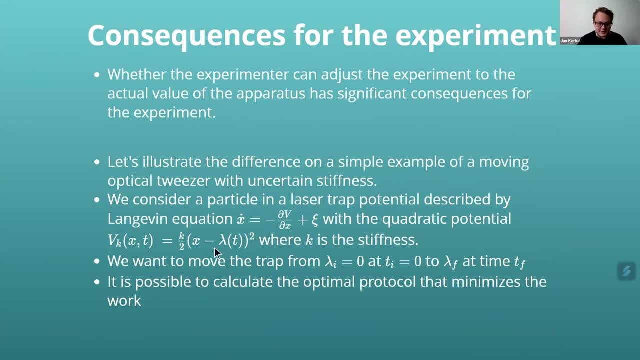 tweezer and the moving optical tweezer has this stiffness function. this is this, basically this quadratic potential, And this k is a stiffness. And let's say we want to move the trap from zero to some finite value, lambda f in time, tf, And we can. 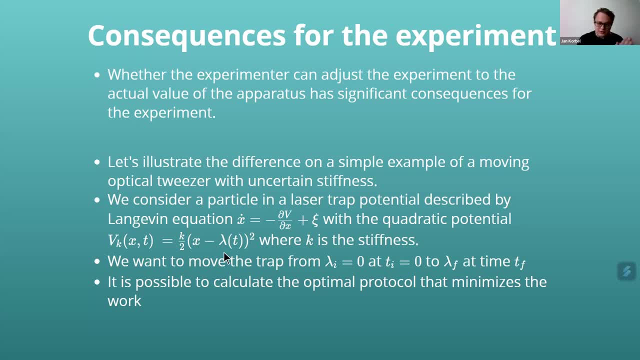 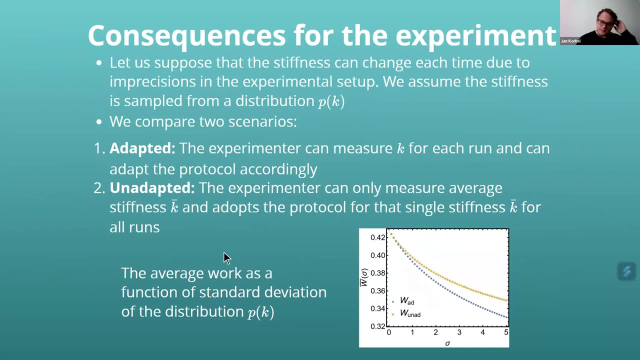 calculate the optimal protocol and everything. Let's say, we choose the optimal protocol so that it minimizes the average work And the problem is that if we know the, if we know the apparatus, if you know the stiffness, then we can change the protocol for each value of. 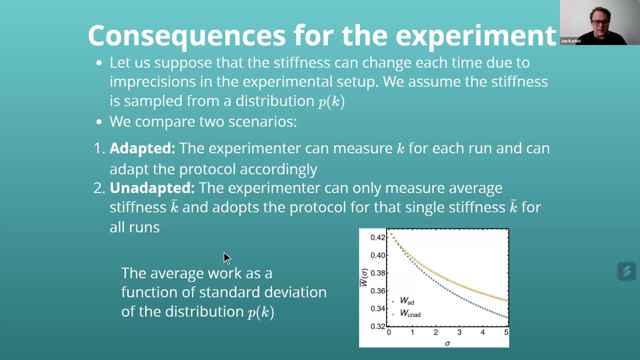 the stiffness. If we do not know this, then we basically measure the stiffness many times And then we, for example, say: let's measure the stiffness of many times and just use the average value that we have, And we think that this average value is. 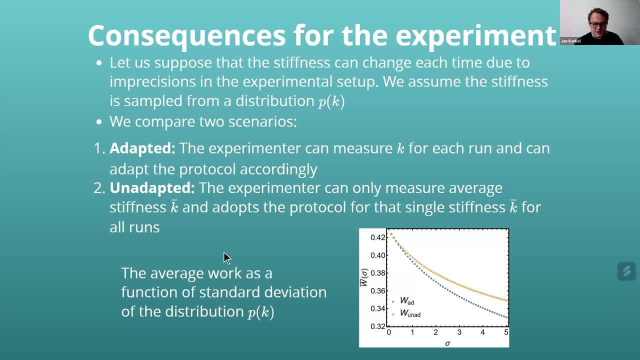 due to the imprecision of the measurement. But the imprecision of it doesn't have to be due to the measurement, but due to the fact that the real stiffness changes in every round, And then one can calculate the work in case of the. this we call it. 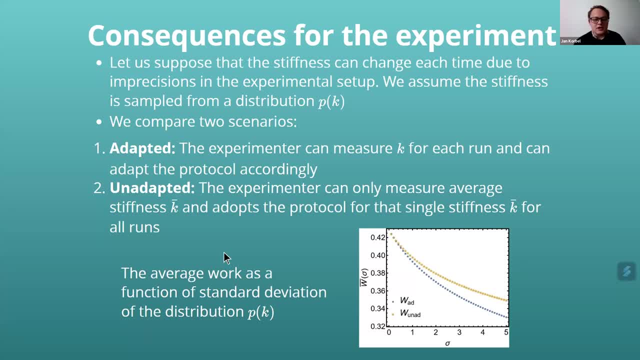 adapted scenario where we can change the protocol for each for each stiffness and unadapted. when we cannot change the protocol and we have to use a single protocol for all cases, And then this is expected, that in this case there is some extra dissipated work that we are spending in this unadapted scenario because we cannot adapt our protocol to the environment. 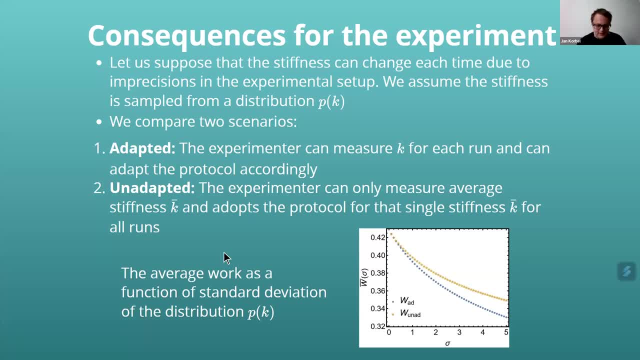 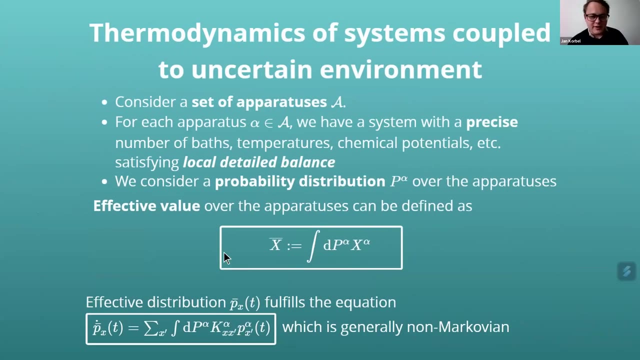 And then the question is: what is then the optimal protocol for this unadapted scenario and how we can deal with these quantities in this case? So let's start with a simple definition. Let's say we have set of apparatuses and here we use this, let's say, generic description apparatus. 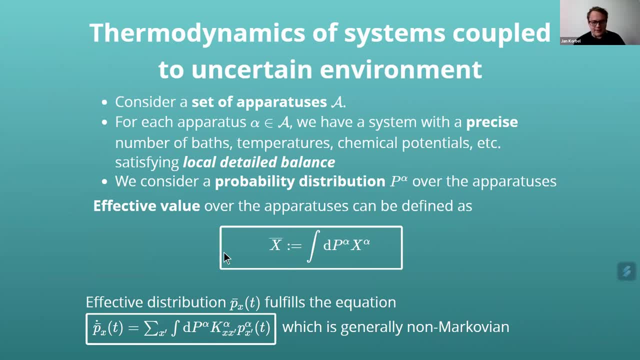 but it can be really set of temperatures, Set of chemical potentials, set of whether it's connected, whether the system is coupled to one reservoir or multiple reservoirs, and all of these details. So the only assumption is that in each case, for each apparatus, let's say that the system satisfies the local detailed balance. 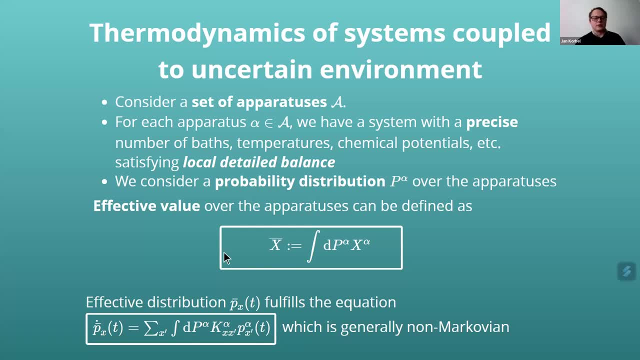 so that we can interpret the quantities from the terminic point of view. And let's say that we consider a probability distribution over the apparatuses, And then, of course, the effective value of any terminic quantity is basically just the average over all apparatuses. 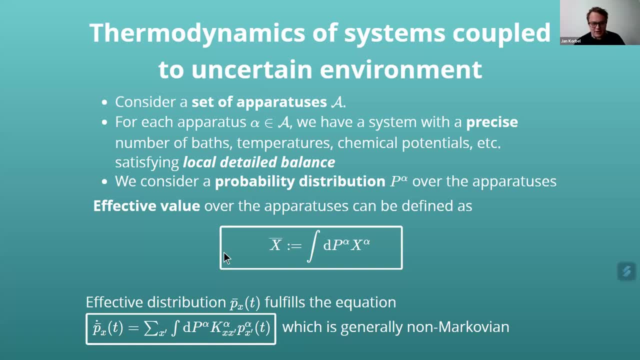 In this case, the effective distribution that can be calculated fulfills this equation And unfortunately this is non-Markovian equation. So this is the first complication in our case, because the averaging over many apparatuses causes that basically there is a coupling between the probability distribution of an apparatus and probability distribution of the system. 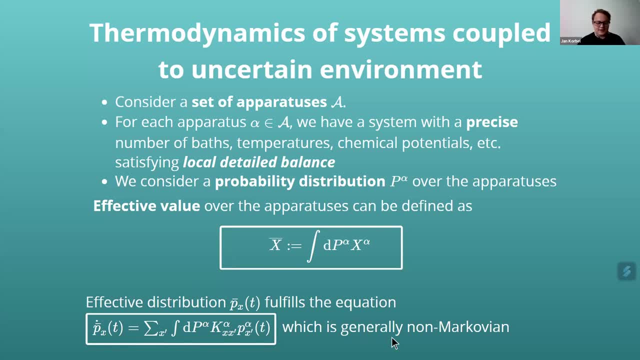 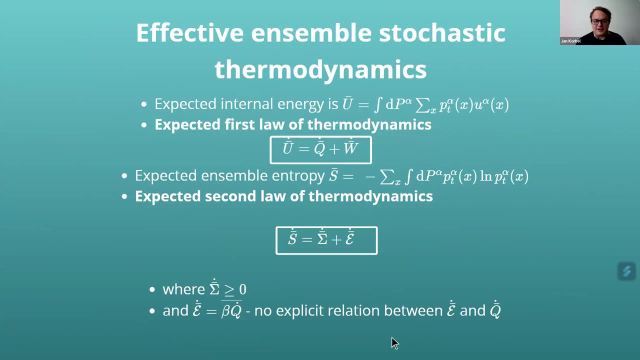 So then the evolution is not anymore Markovian. in this effective case We can investigate the first and second law of thermodynamics. The expected first law of thermodynamics is as expected. So basically, the change in the internal energy, the effective change, 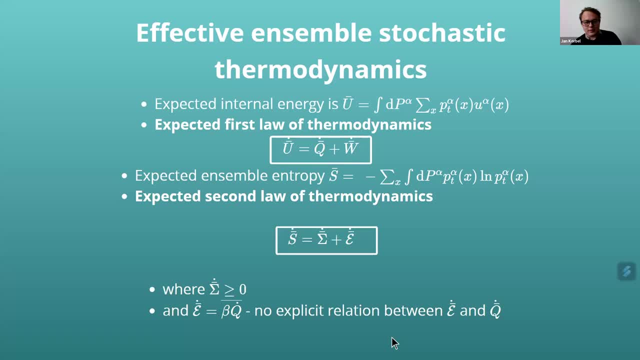 is equal to the effective change of the heat and the effective change to the work. Then for the kind of second law, or let's say the decomposition of entropy into the entropy production term and entropy flow term, this still works. So there is this expected entropy production. that is not negative. 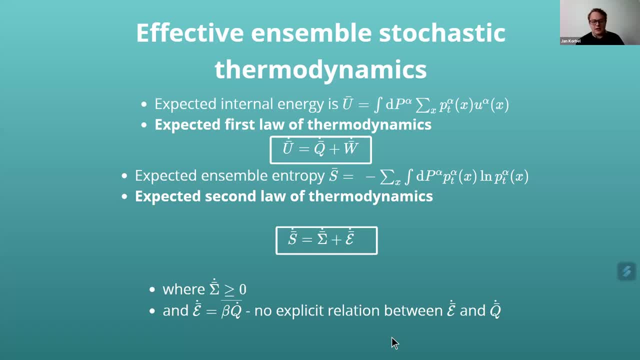 The problem is that the expected entropy flow that is normally equal to the inverse temperature times, the heat flow, is not valid, Because the expected entropy flow is the average value over the beta times, the Q which is. this is just for the case of one heat bath. 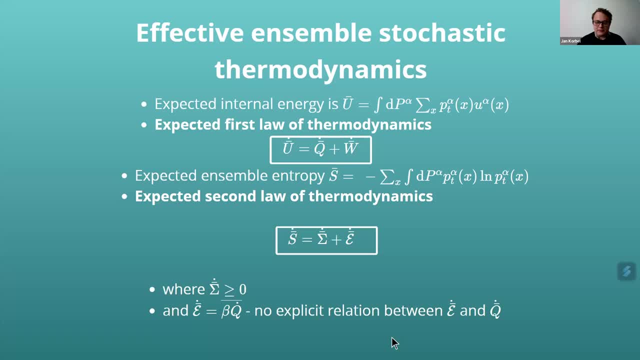 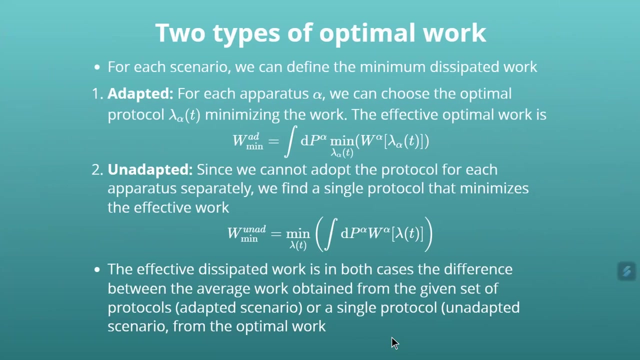 So there is no explicit relation between the entropy flow and the heat flow, which is the cornerstone of the second law of thermodynamics. So here the thermodynamic description or interpretation is a little bit more complicated. Okay, So now we were talking about these two scenarios. 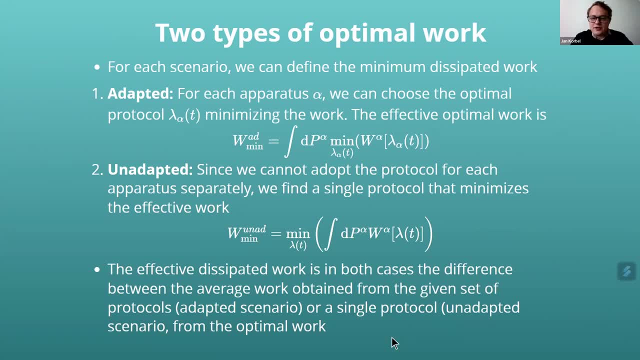 So basically, for the adapted scenario, for each apparatus we can choose the optimal protocol that minimizes the work. So basically, then, what we do is that for each apparatus we choose the optimal protocol that minimizes the work, and then we average. 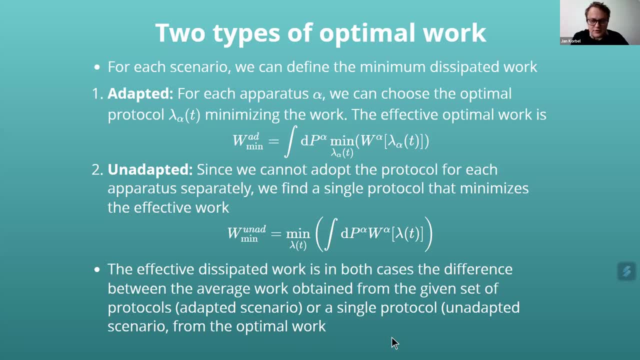 And for the unadapted. unfortunately, we cannot do that. We have to use the single protocol And, of course, the difference between these two things is telling us what is the difference between the work in the unadapted scenario and adapted scenario. 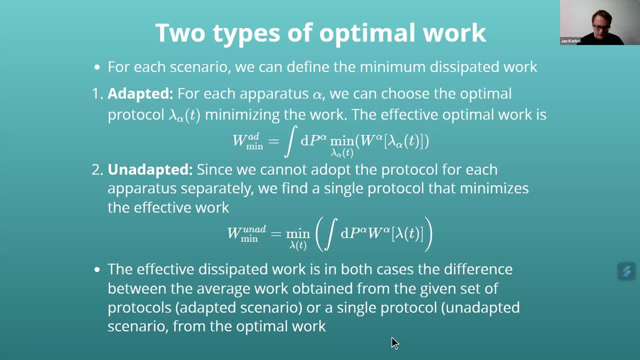 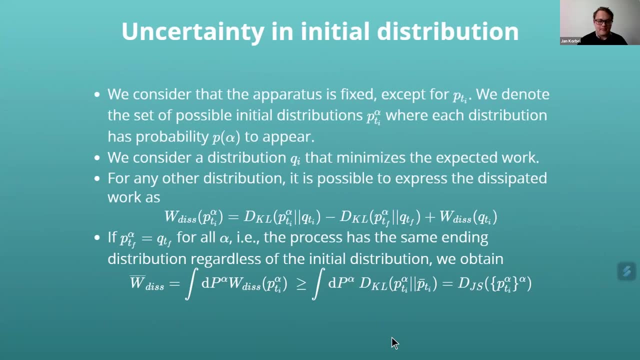 And basically this is what we can call an extra dissipated work due to this lack of knowledge of apparatus. Let's now just focus on a very specific scenario, because one of the uncertainties that can be is just the uncertainty about the initial state. 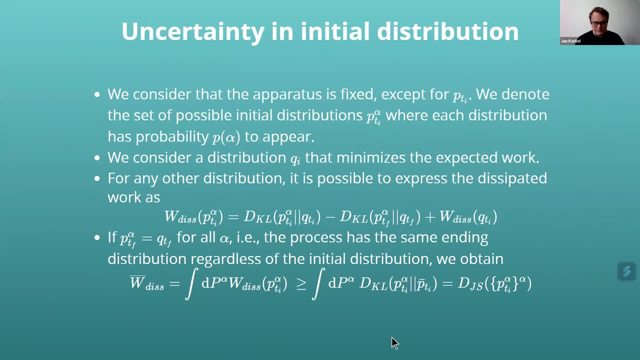 So let's say that everything is fixed, Everything is known. Temperatures are known, Temperatures are known, Chemical potentials are known. Everything is known except for the initial distribution. And let's say we have a set of possible initial distributions and each distribution has some probability to appear. 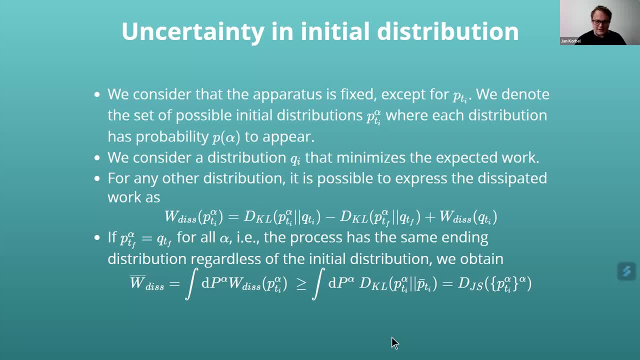 And let's say we have a distribution that minimizes the expected work, and then we know that any other distribution, for any other distribution, there is a formula for the dissipated work that is the minimum dissipated work done by this optimal distribution. 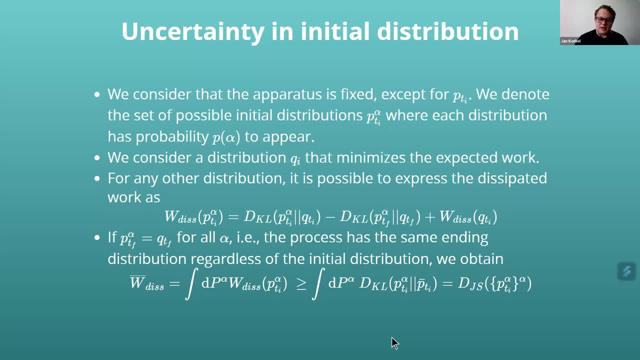 And there is this drop in the scale of divergence which is called mismatch cost. that basically tells us what is this difference between the dissipated work for non-optimal distribution versus the optimal distribution, And one can show quite a nice fact, quite interesting fact. 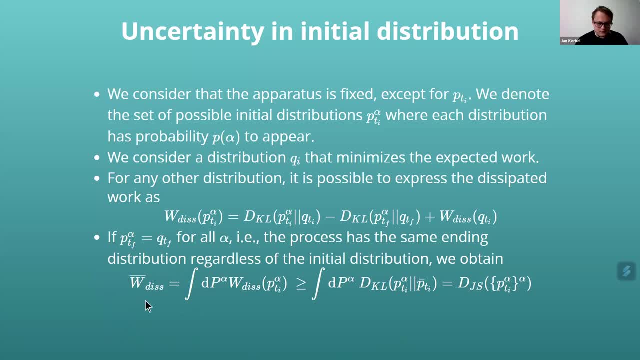 that this average dissipative work- dissipated work in the case where we average over the all possible initial distribution- can be calculated as a so-called Janssen equation- Janssen-Shannon divergence- where we basically take all the distributions. 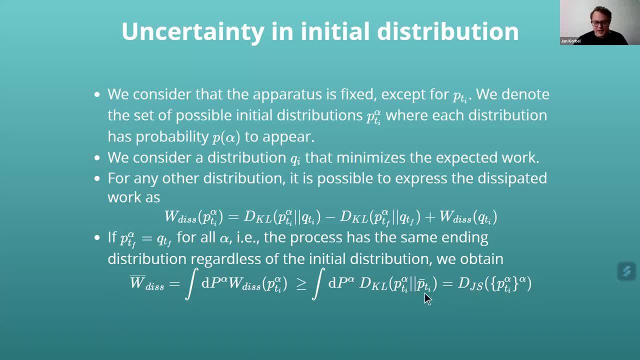 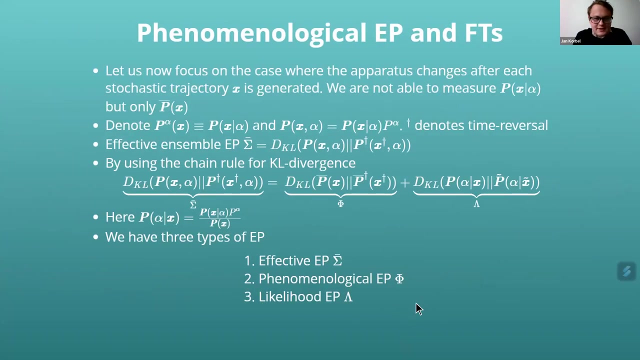 weight them by their probabilities, and this is the KL divergence that takes as this null model the average distribution. So then we can easily calculate the dissipated work. that is just this Janssen-Shannon divergence. Last thing I want to talk about is the way that it also 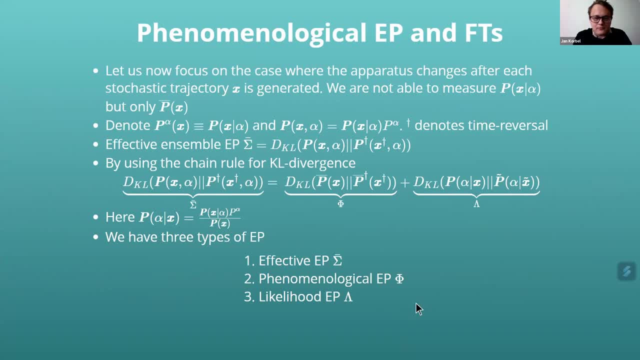 in this case we can formulate some fluctuation terms and we can also decompose the entropy production into two interesting terms. So let us now just basically say that we are in this case of phenomenological approach, where we cannot measure the probabilities for each apparatus. 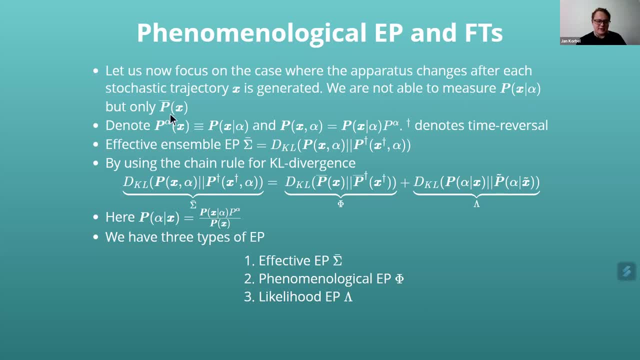 particularly trajectory probabilities, but only the probabilities averaged over all apparatuses. And here we denote the trajectory probabilities as follows: And of course the effective ensemble and production is the KL divergence between the forward probability of the trajectory versus the backward. This is the standard result. 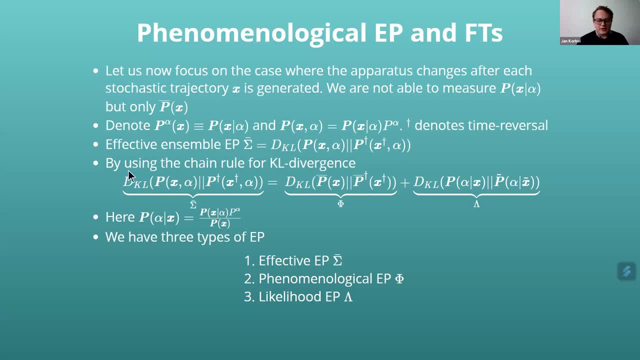 And by using the chain rule for KL divergence, we can show that this can be decomposed into two terms. So this is the KL divergence over the average probability of the trajectory with respect to the average backward trajectory, And there is a term where the role of this X and alpha is changed. 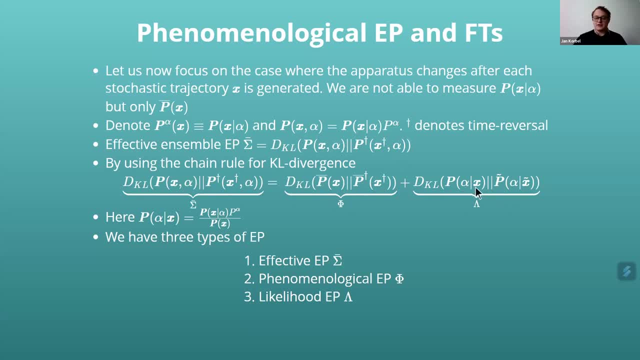 So it's the probability of observing alpha, given the trajectory. And basically we have now the three types of the entropy production. So one is the effective one, One is the phenomenological one. So this is the effective that is averaged over all apparatuses. 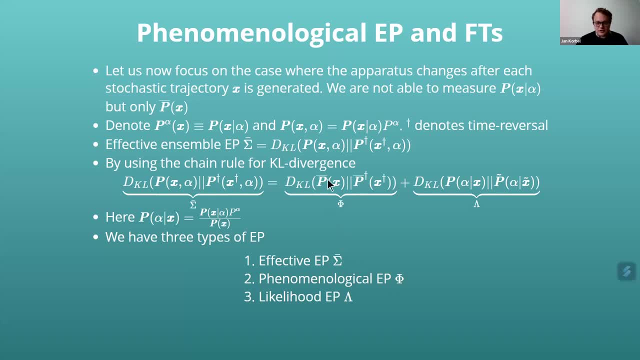 This is the entropy production over the average trajectories, And this is something that we call likelihood entropy production. And if you look at it, it's interesting to see that here, in this case, you don't calculate the probability of the trajectory given the apparatus. 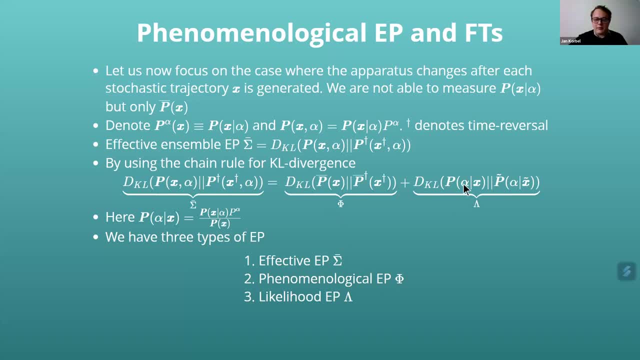 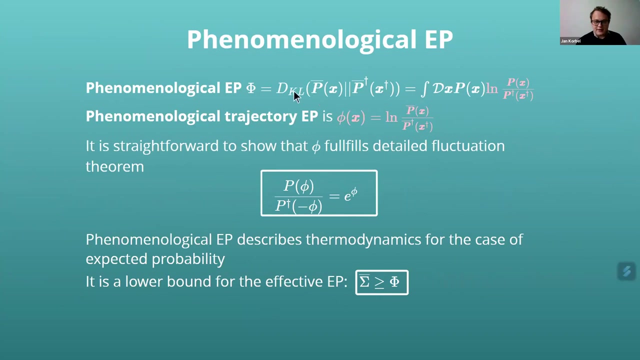 You are calculating the probability of the apparatus given the trajectory. So basically you do the reverse thing. So you are learning about the apparatus from observing the trajectory And, in the case of phenomenological entropy production, you can basically rewrite the express, the KL divergence of this. 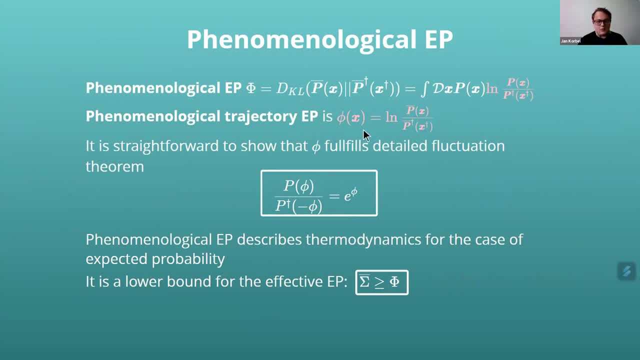 And in this case you get the trajectory entropy production, which is simple to show that it fulfills the detailed fluctuation theorem And of course, the conclusion from this is that this phenomenological entropy production is the lower bound of the full effective entropy production. 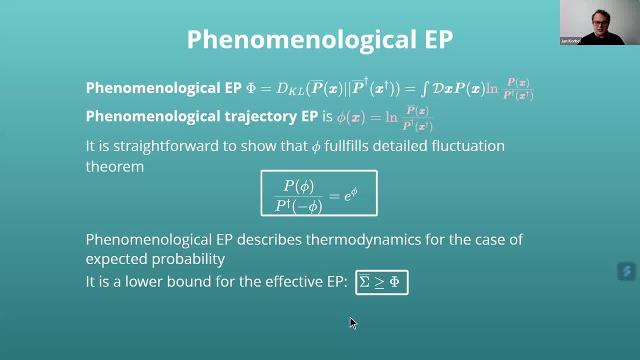 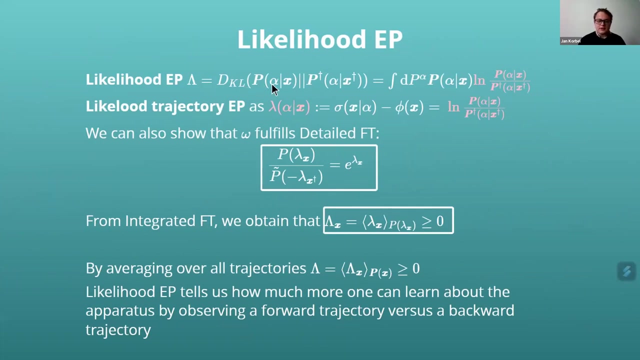 So by observing the only the average trajectory probabilities over the all apparatuses, you can estimate lower bound of the effective entropy production. And for the second quantity, this KL divergence or P alpha, given X, you can also calculate the likelihood trajectory of entropy production. 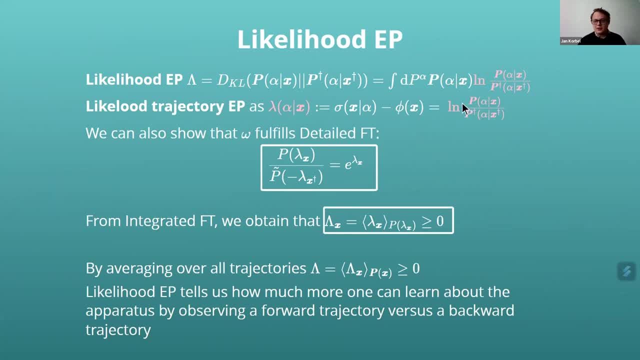 And if you look at it it really looks like- look like likelihood function that you are trying to calculate the probability of parameters given the trajectory. So this is your data and this is this is your parameters, And then again it fulfills a detailed fluctuation theorem. 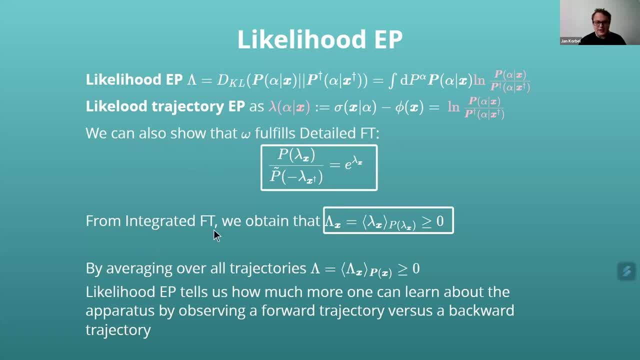 And interesting is that from integrated fluctuation theorem you get a result that the average Lambda- this is the average trajectory- entropy production- given the trajectory is still for one trajectory- is larger or equal one. What it means is that, basically, the detailed fluctuation term tells us how 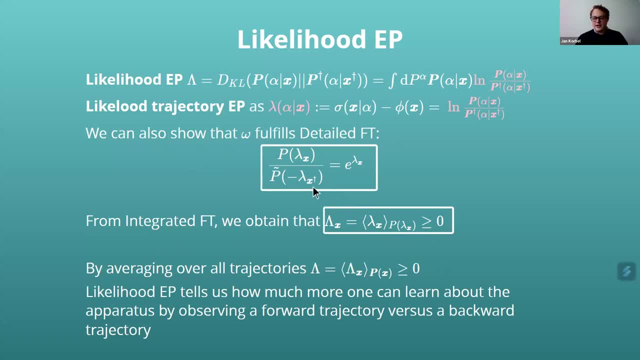 much we learn from observing the forward trajectory versus learning from, versus how much we learn from observing the uh, observing the backwards trajectory in the in the backwards scenario. So, basically, uh, it's uh determining um the difference between observing the trajectory forward. 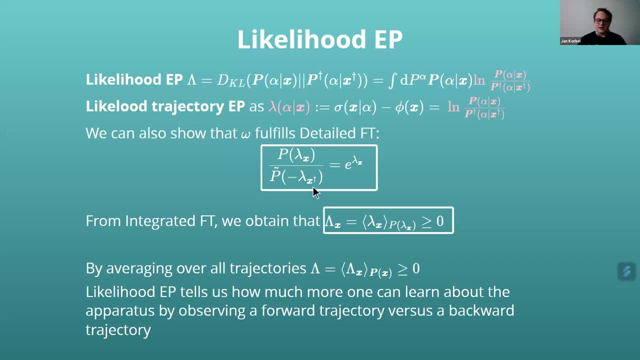 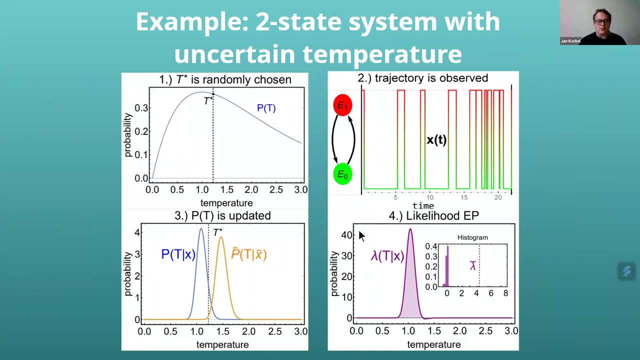 learning from it and observing the trajectory backwards, learning the parameters from it. Uh, this is one example how it can be calculated. So, basically, if we have, let's say, a distribution of temperatures and we have a simple system of two states, then basically we observe a trajectory and 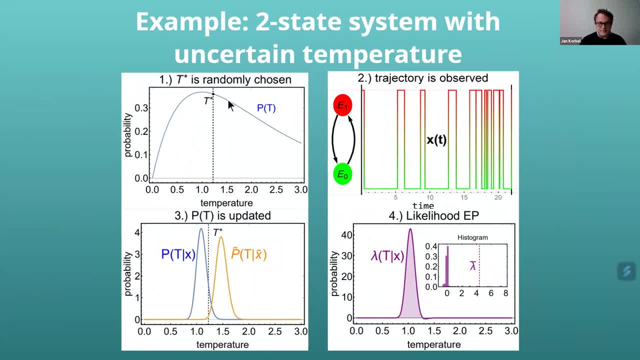 um, this is, this is uh sampled from uh some unknown temperature, So we can then uh update the, the um, the, the probability of temperature observing the trajectory X. Let's say that the the 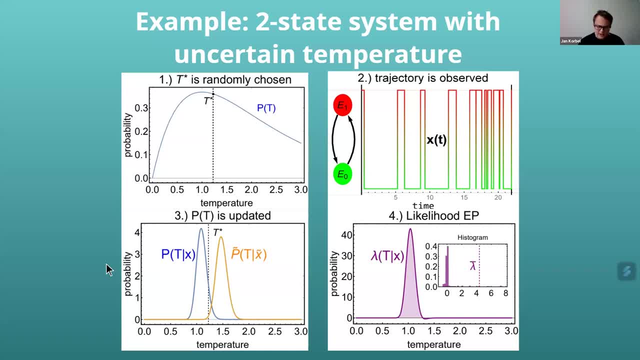 uh. prior distribution over temperatures is uniform from this zero to three. And then by observing this trajectory, we can calculate the probability of observing T, given the forward trajectory. This is the uh. uh probability of observing the temperature. uh. 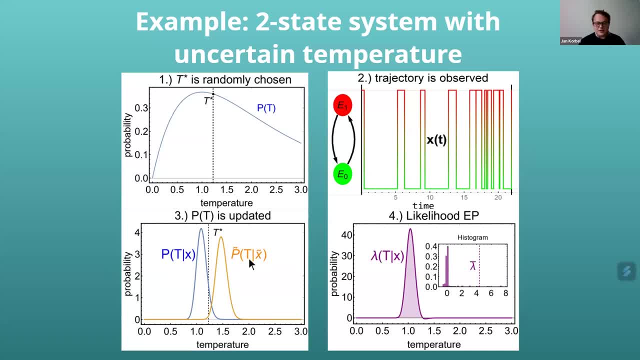 given the backwards trajectory, I can calculate likelihood, entropy, production, And this is again given the X. and you see it, for some temperatures there is a slightly negative value, but uh, if you calculate the overall value it's positive. So here it's. 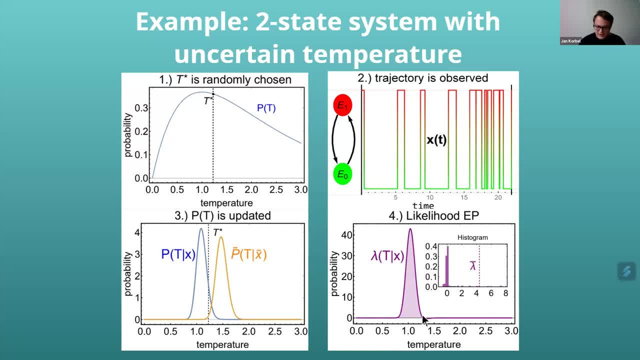 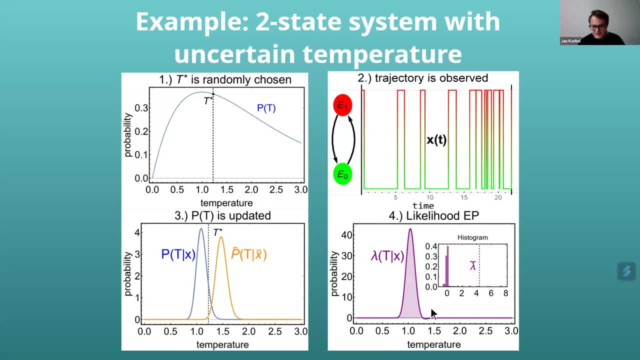 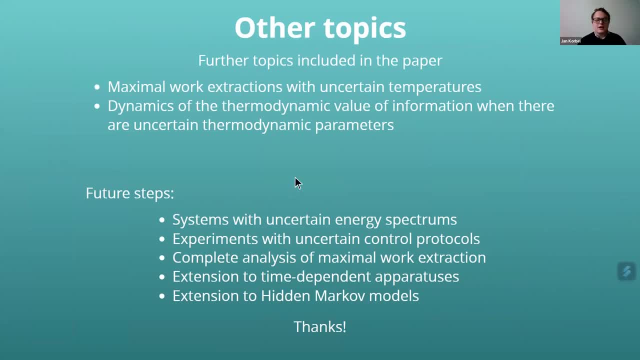 cases where some temperatures where it is smaller than zero, but it's it's. it's just a small region And I just want to say that I didn't have time to go through all of the details that are, uh, or all of the results mentioned in the paper. 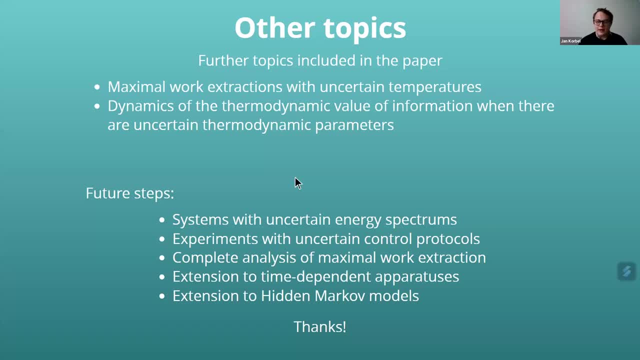 There is also a section on maximum work extraction with uncertain temperatures. also dynamics of the thermodynamic value of information When, the when there are some uncertain thermodynamic parameters- and there are. this is just a very first step to uh, the whole. 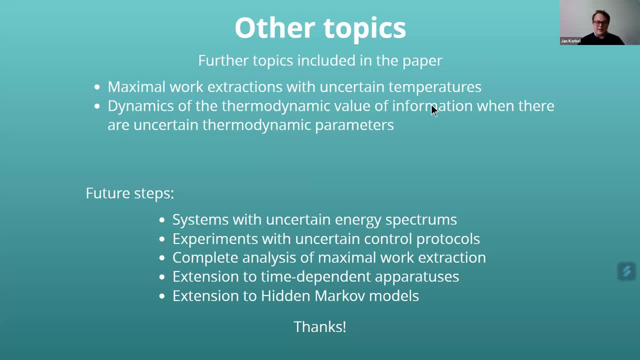 uh new field of uh: processes with um- uncertain um environments, uh where you can consider systems with uncertain energy spectra, experiments with uh- uncertain contour protocols, uh extension to time-dependent apparatuses. So basically, then you say that your temperature. 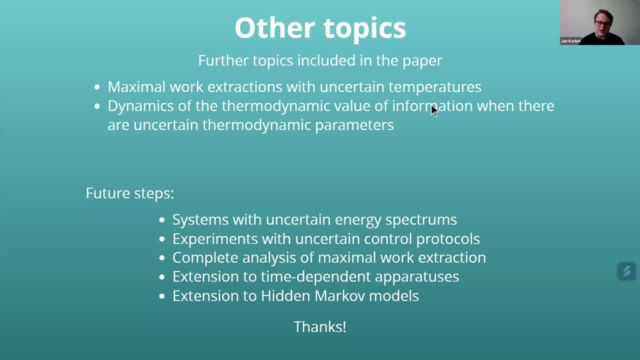 your temperature can change in time, but you don't know how you can have some uh probabilistic equation on that And you can maybe try to uh calculate uh trajectory probabilities of these temperatures and other things. Also, extension to a hidden Markov models. 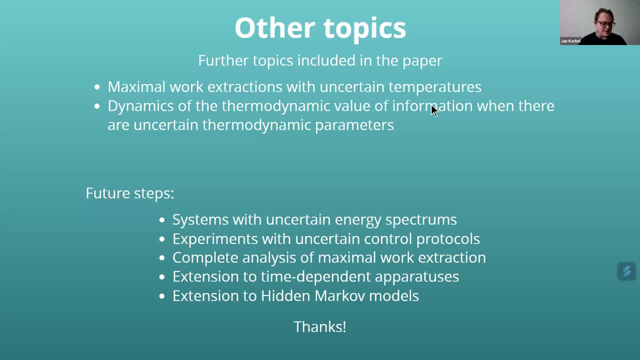 That would be very convenient for several uh systems. And that's basically all uh from me, So thank you very much, And now it's time for questions And I will try to uh open the list of participants. 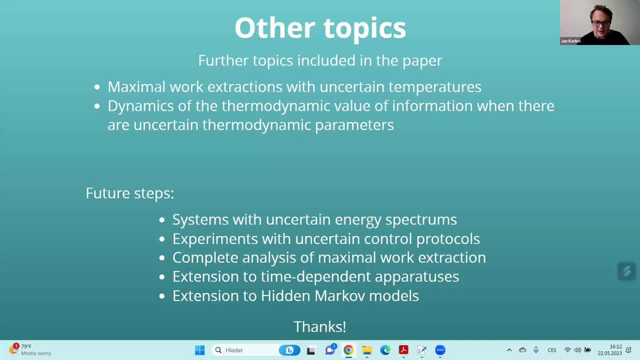 And please raise your hand if you have a question. Yes, Uh, you're not done. Hello, Um, thank, thank you for the very wonderful talk. Um, I, I see at the end you're talking about, if you have. 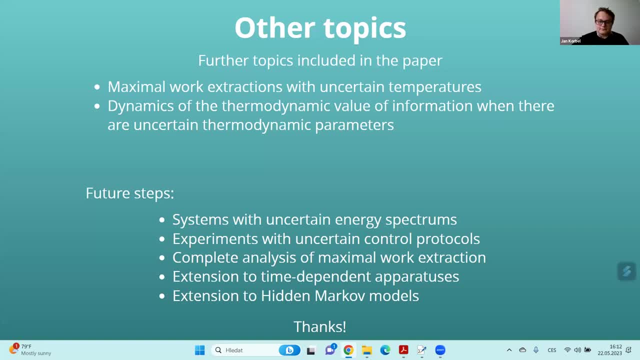 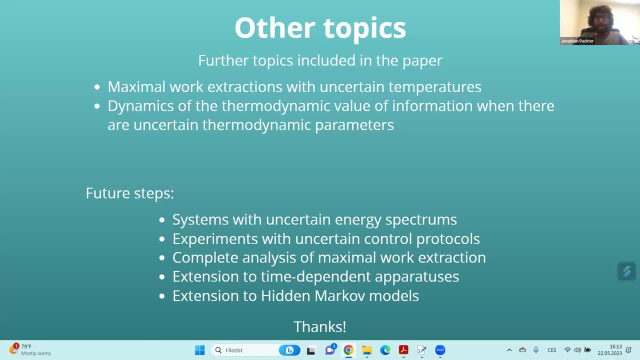 parameters that not only are the uncertain fluctuating in time, but but they themselves are affected by the dynamics of the system, or there would be some sort of feedback between the two of yeah, That that will be another interesting step here. I just want to mention that basically. 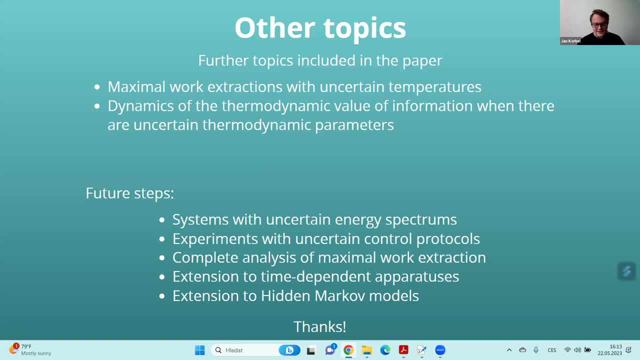 mention that basically, the difference between all of these great field of, let's say, time dependent temperature or time dependent parameters is the fact that here we consider that we there are fixed, or can be maybe even time dependent, but we do not know the exact values. so in this case, 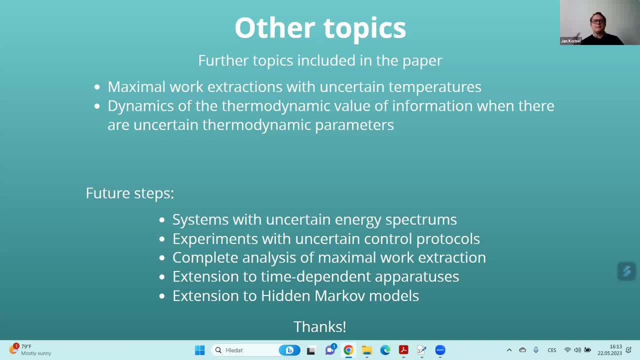 there would be another great, basically great- interplay between the system and the environment where you just know the part of the environment, like the part of that is your system, and you have only some information about the environment and there can be some, uh, some, some feedback loop for. 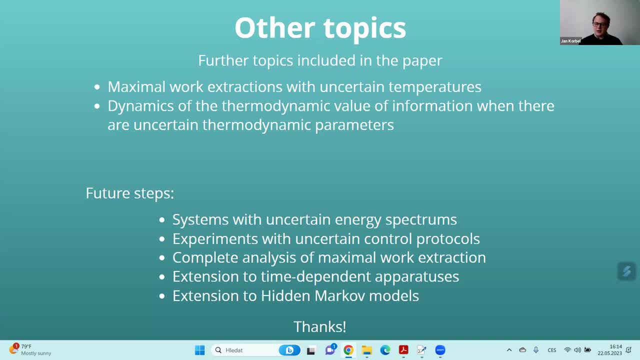 example in this. you haven't considered that? that would be great. uh, future step. thank you very much. thank you, uh. are there some more questions? i could have a? i would have a question. yeah, peter, um, so you show these two scenarios, um, all right, one scenario, the adaptive scenario, where you know, you measure alpha, you know what. 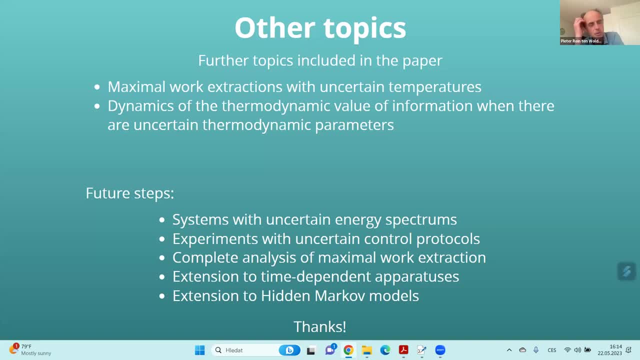 it is, and then you carry out the optimal protocol for that. and the other is where you only uh know the average, do the work, uh extraction for the average. but i was just wondering. so suppose that you know the distribution of alpha and then you do your experiment. uh, to extract work, for example, is then, but then you're only allowed to. 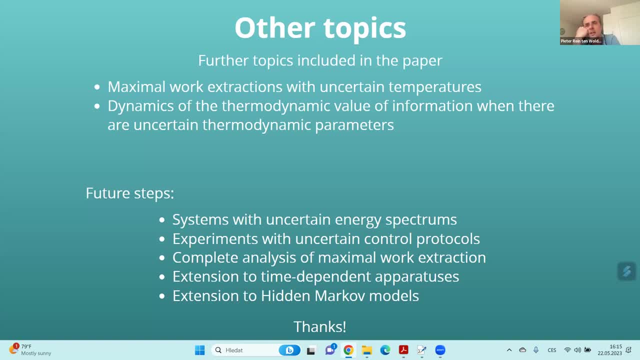 choose, let's say, one alpha for each. Let's say alpha gives a certain temperature, and other times you can go to the observable one for the continue effect from that distribution. what would then be the optimal alpha? is that necessarily the average, or i guess, yeah, so, uh, so that's that's the. that's the thing, so that, uh, what we see typically is that. 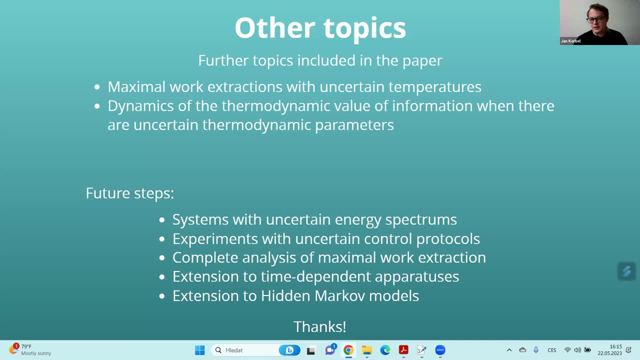 choosing just the average is not the optimal. it's not the optimal one. also, uh, it's true for the protocol and i didn't have a time. uh, in the paper we have a simple example of a bit erasure, where you basically couple the system to a bath of of uncertain temperature and then you choose your. 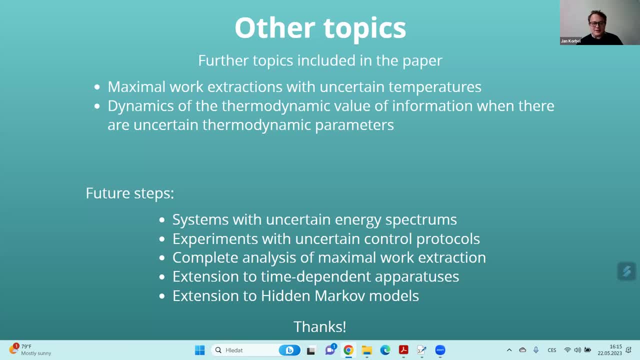 protocol. that erases your bit. and then it shows that the protocol is not simple average of the two protocols. also, it's not, uh, average of the temperatures or something like that. it's really very complicated and in general very difficult to find. yeah, i can, i can understand. yes, thank you. 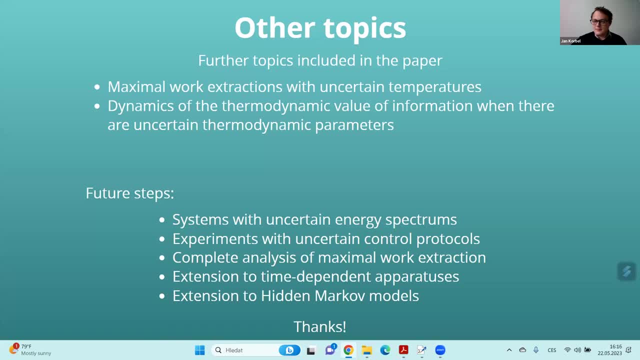 yes, yep, um, are there some more questions? yeah, maybe i can also mention that that there will be also next interesting step, where you don't know the protocol. you observe the trajectory, you try to estimate the um, the apparatus, and then you try to change, adapt the protocol. uh, regarding to your information, you gain from observing the 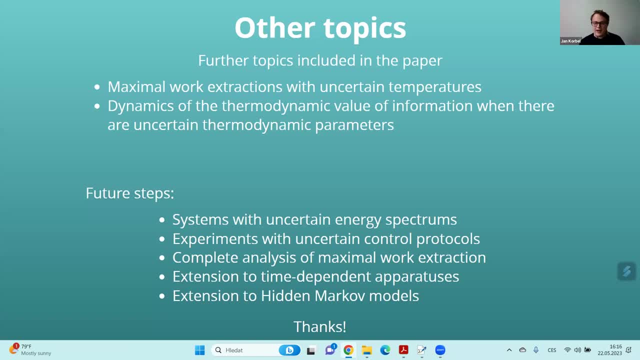 trajectory and then you try to change, adapt the protocol, uh, regarding to your information you gain from observing the trajectory and in this case you would have the feedback loop. and then there would be a natural question: what is the, what is the trade-off between observing the trajectory? 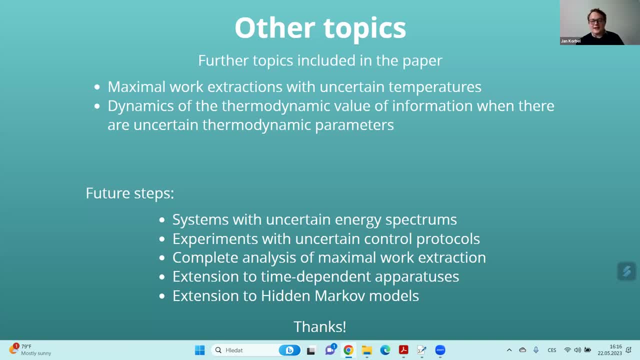 and changing the protocol and this well-known exploration versus exploitation problem from reinforcement learning. that would be great. next, next step. so, um, exactly, uh, rohit was the next one. yeah, my question is, uh, pretty simple. i didn't understand how you got the non-markovian feature through averaging in the beginning, when 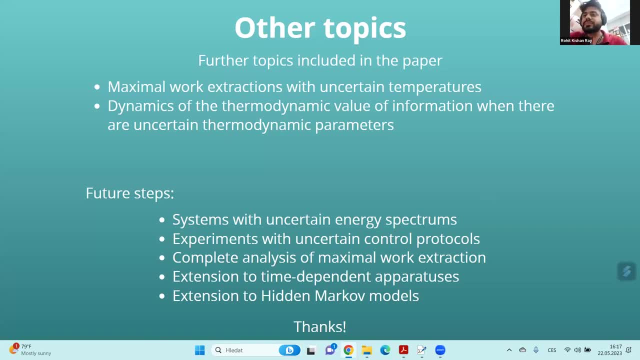 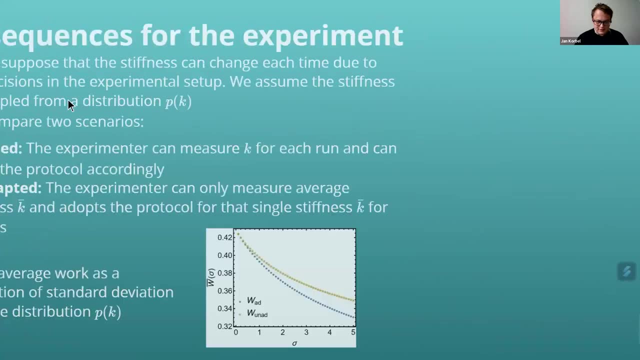 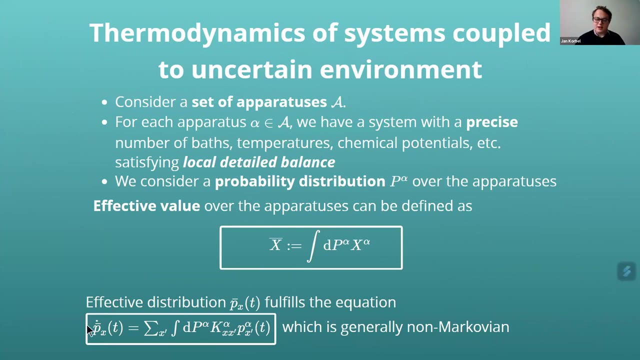 you were averaging over the effects of all the apparatus. yeah, that's, that's the problem, that, basically, if you look at this, at this equation, then if, if this equation would be uh, markovian, it would be uh, on the right hand side, you would have some function, some, some transition matrix. 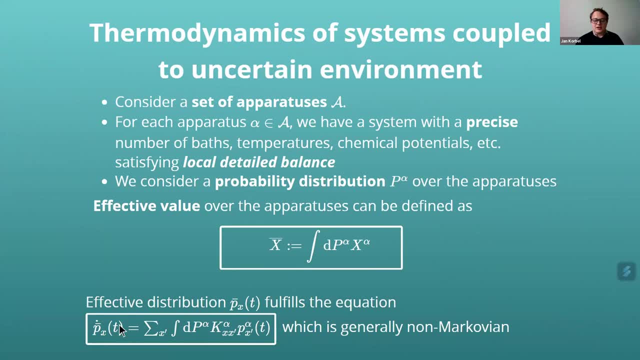 some rate matrix time the average uh distribution. unfortunately, you cannot decouple this integral into the product of the some rate matrix times the average distribution. so basically, the simply said: the integral of a product is not the product of integrals and that's why you get this non-markovian, non-markovianity in general. okay, okay, thanks, okay so. 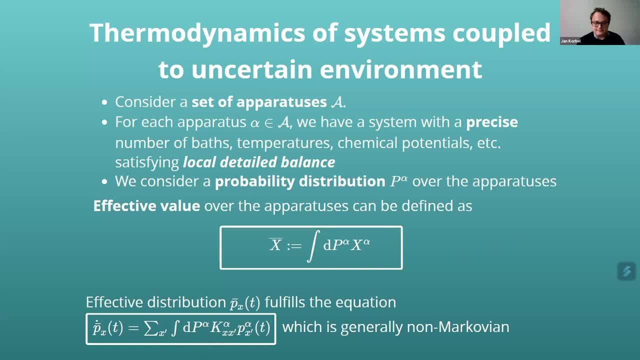 so next question by Sangella Chen. hi, my name is Sangella. thank you for the talk. could you repeat: um, what was the what? what are the apparatuses? are they just different baths that you can couple to? yes, yes, so so we had this, this abstract term for any kind of parameters that you have. it can be. 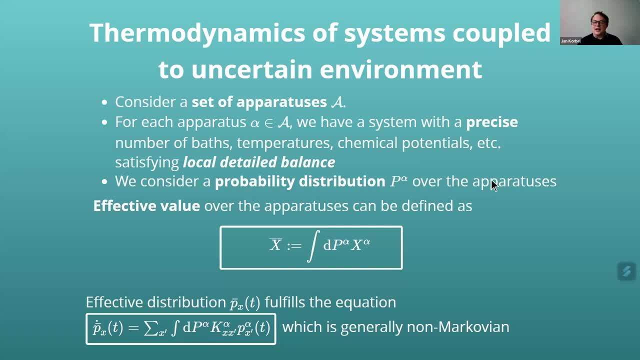 temperature of a bath, it can be chemical potential, it can be even the stiffness parameter, everything that is a parameter of your experiment. So then I'm a little confused about what the protocol entails. Is it just like choosing different? So if an apparatus is some parameter, then you're choosing different apparatuses? 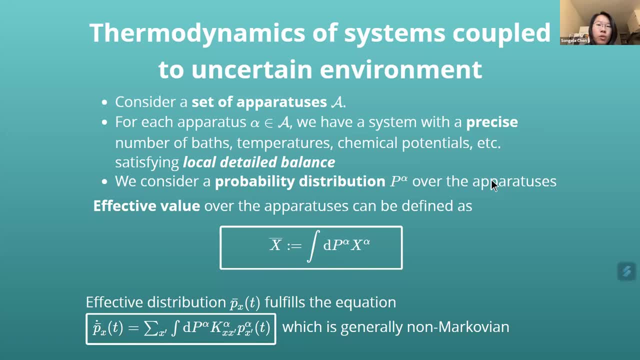 meaning you're choosing different parameters in some order, and that's what you call your protocol. Yeah, and in this case, the protocol means changing the energy spectrum so that you do what you want, And, of course, you do it in some way depending on the parameters. 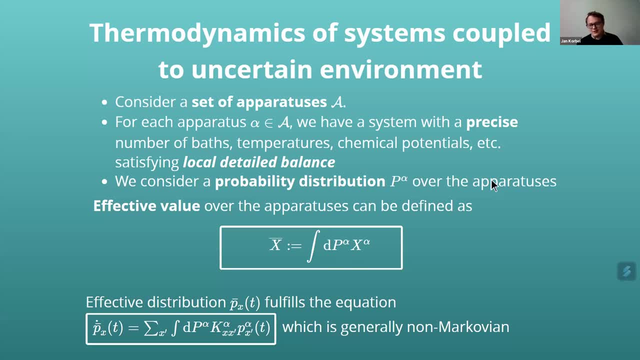 but if you do not know them, you have to somehow deal with all of these scenarios that might happen. Okay, thank you, And okay, and the last public question by John Hi, yeah, thanks. So, if I understand, the uncertainties that you're considering are all parametric. 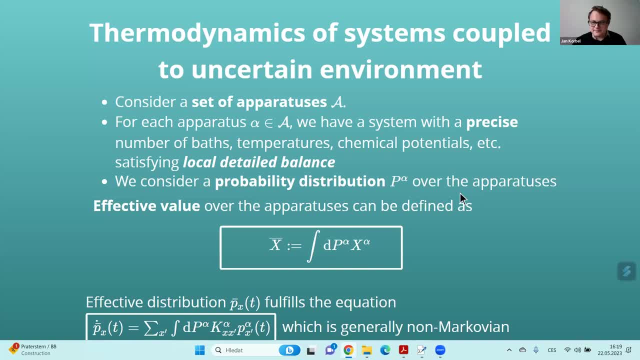 in the sense that I have a stiffness of a potential and I don't know, Have you thought about kind of less structured types of uncertainties? Like maybe I have a potential and it's almost parabolic but differs a little bit in shape? 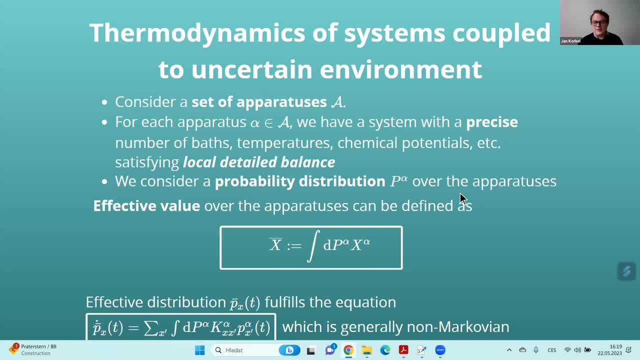 Yeah, yeah, sure, sure, Yeah. so, for example, you have a class of potentials and they are parametrized. I mean, at the end of the day, it's always that you can parametrize them somehow, or this is the typical approach- that you somehow label them if you want. 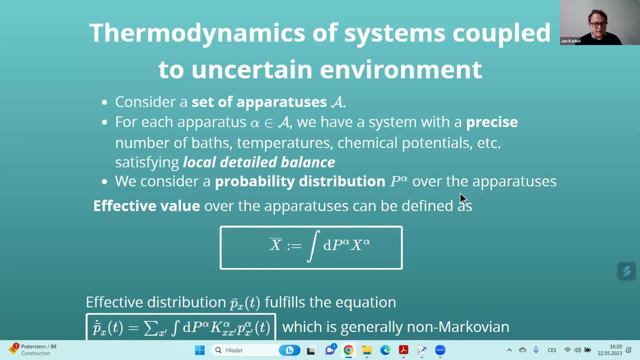 and in our case it can be discrete, it can be continuous, both of them. So basically, you have some set of these, let's say, potentials or apparatuses, and then you somehow average over them, And this goes a little bit into your direction of stochastic control protocol.